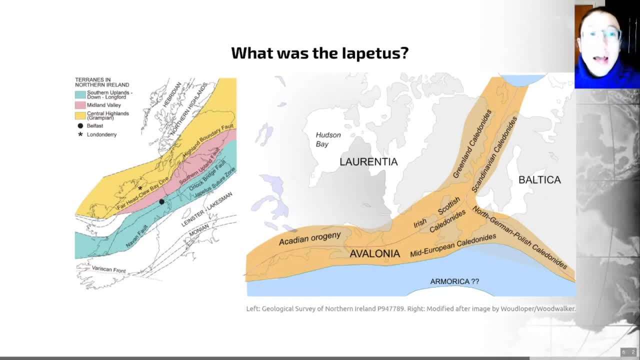 based on paleontological data. so fossils and fossils remain critical to understanding continental movements in deep time. As you can see from the map on the left here, the UK is actually made up of a series of different chunks of old continents. These are things that are called terrains in geological speak. 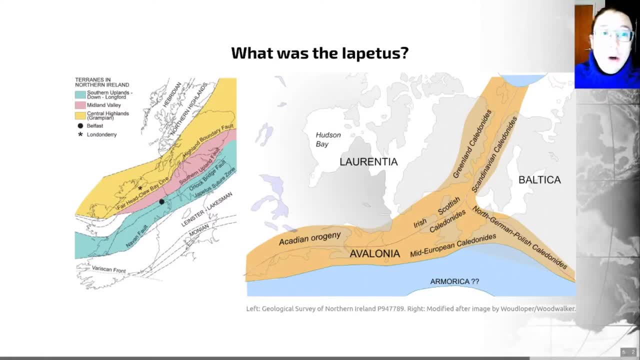 many of which have been identified in part through the fossils that are preserved in them. To illustrate this point, we'll learn a tiny bit more about the Iapetus Ocean, But first I want to quickly mention a tiny bit of history. During the 1960s, as plate tectonic theory was, 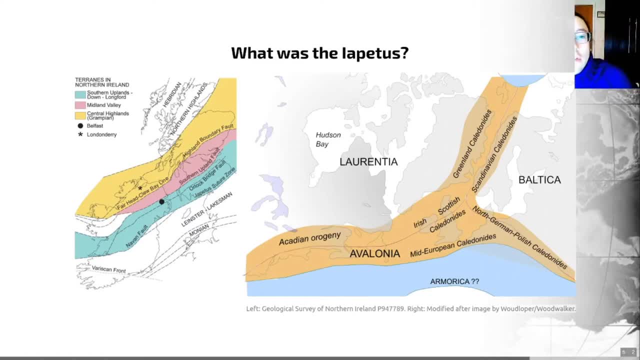 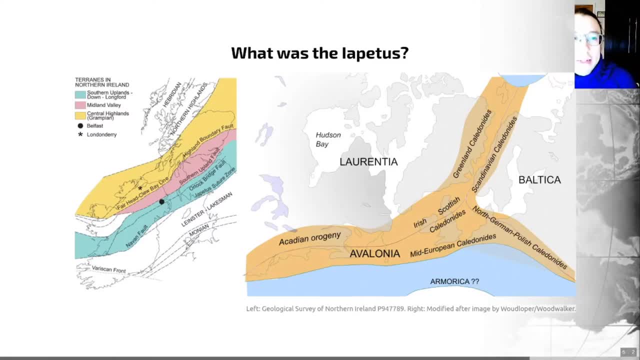 and geophysicist prediction that they were remain for an ancient, ancient seaway would be found in the lower paleozoic rocks of the northern hemisphere. So Wilson used as evidence to support this North American and European fossil assemblages, so assemblages of 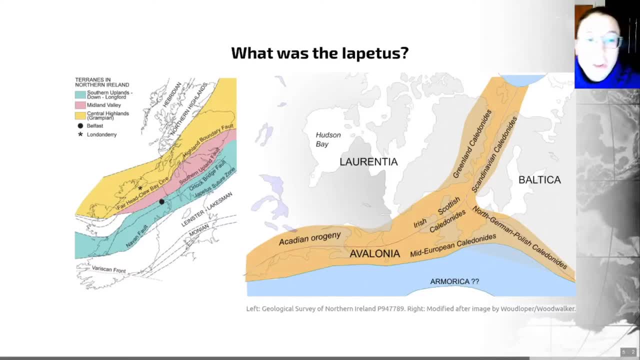 brachiopods, trilobite and grad light species, And he showed that these were separated by a major suture that runs along the length of the modern Appalachian and Caledonian mountain belt. you can see us positioned about two feet away. and what we've down here with this? 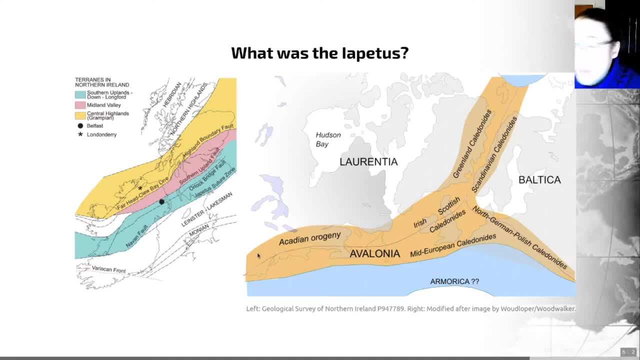 see this suture of this ancient, now closed ocean running throughout modern day Scandinavia, UK and North America. This allowed Wilson to infer the existence of an old ocean, a thing called the Proto-Atlantic, which we now call Iapetus, And he made the argument at this time that this ancient ocean separated North America. 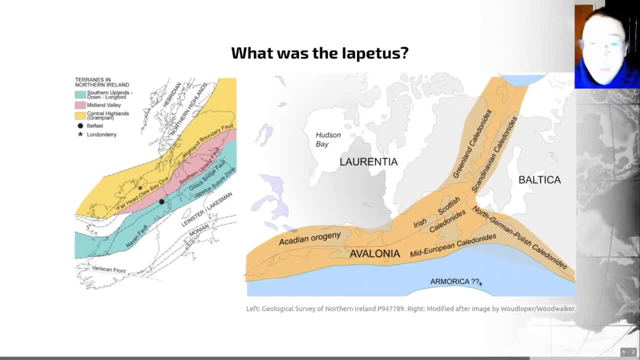 and these tiny bits of Europe up here from the remainder of what is now the European continent until there was a collision of these continents and an oceanic closure. that happened in the Silurian and the Devonian periods. So I'm going to give a quick introduction to this over the course of this video. but 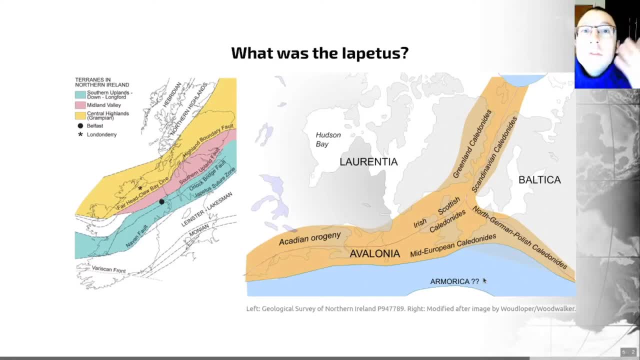 I will do so focusing on the fossils. Bear in mind that evidence from fossils is supplemented by, for example, evidence from paleomagnetism, Rock facies, glacial lithologies and lithologies associated with mantle plumes. All of these lines of evidence have been used to build the picture that I'm about to be. 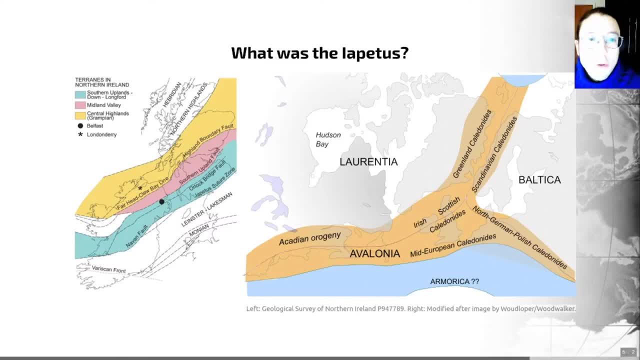 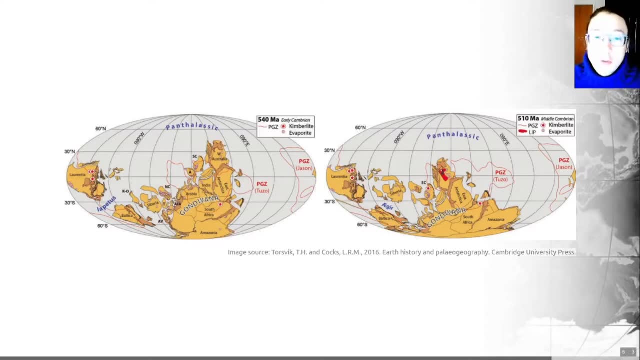 showing you, despite the fact that my focus will be on the fossils. I'll start by giving you a very quick overview of the history of this ocean as a whole before diving into a bit more detail with my next couple of slides. The Iapetus Ocean is shown on this paleogeographic reconstruction from 540 BC. 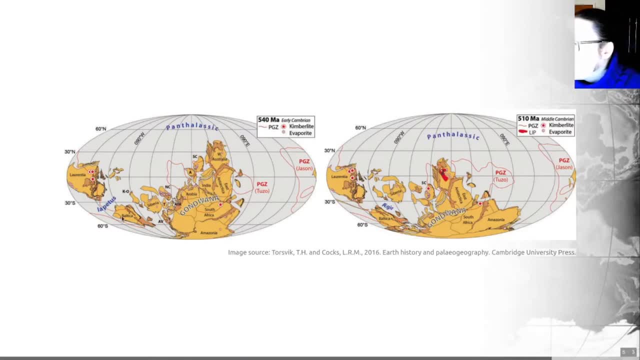 This is the Iapetus Ocean. This is the Iapetus Ocean. This is the Iapetus Ocean. A ballad appeared at the final point of the Iapetus Ocean 40 million years ago. You can see it here, between an ancient continent called Baltica and an ancient one called Laurentia. 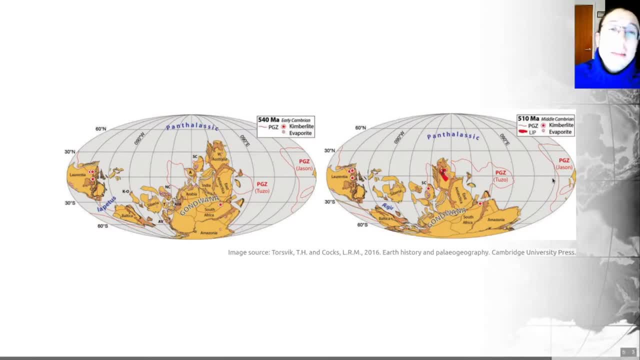 More on that in the next slide. The Iapetus Ocean actually first opened during the Late Precambrian. It followed the break-up of a supercontinent called Redinia. It developed throughout the Cambrian and reached its widest extent in the Late Campseat- a little. 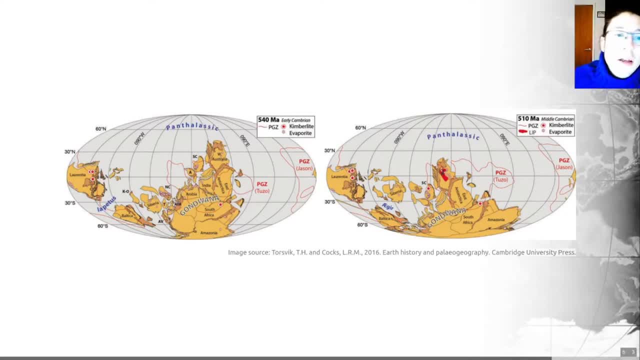 bit after this paleogeographic reconstruction here, much as 4,000 kilometers across at its widest. We can surmise this because only pelagic taxa, in this case floating graptolites, were similar on both sides of this ancient ocean, But then over the next tens, to hundreds of millions of 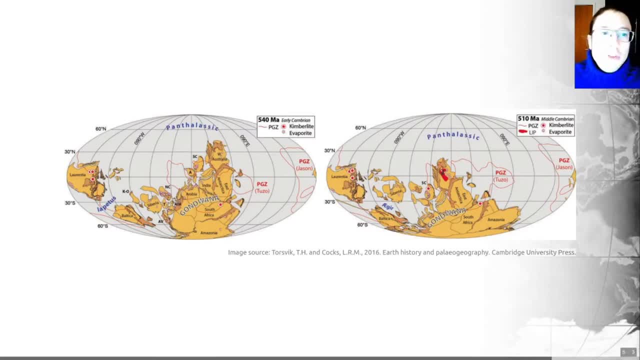 years this ocean closed. First we see swimming organisms, for example. there's a group of organisms that are closely related to modern-day vertebrates, called the conolonts, that could cross this seaway, And later we start seeing both the mobile and, eventually, the sessile, or fixed benthic communities of this time. 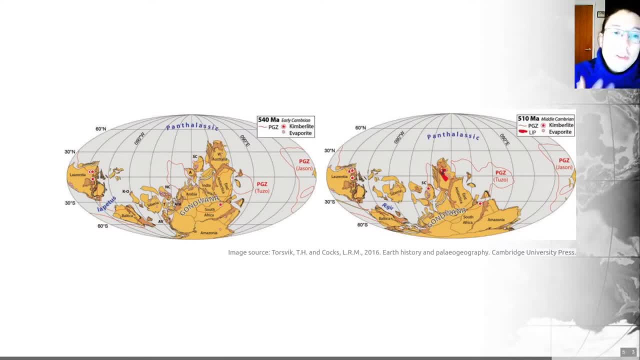 that include trilobites and brachypods, crossing this seaway as it got narrower and narrower, Indeed by the late Silurian. as the Iapetus narrowed to only a few hundred kilometers, we start seeing even tiny creatures like the benthic. so that's some seafloor-dwelling ostracods. These are really tiny creatures, crustaceans, that don't really travel that far. We see them managing to cross this ocean by the late Silurian And by the Devonian. the ocean was almost. 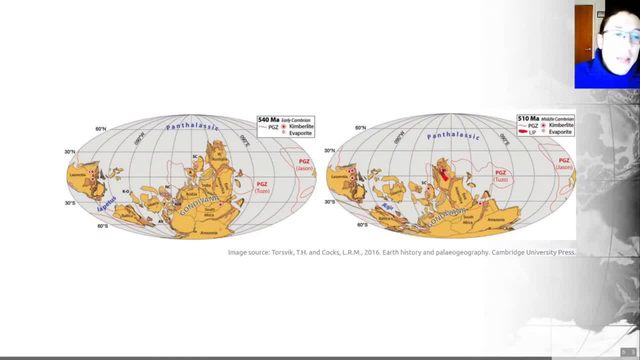 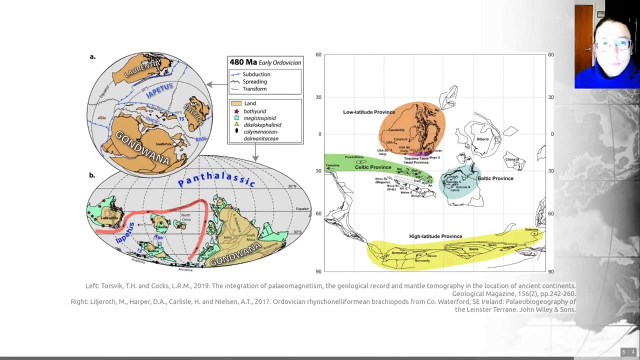 completely closed and freshwater fishes were similar in both Europe and North America. So basically, this has created a single continental mass by that time period. So that's a nice story. How can we use the fossils to unravel that story a bit more? and what do they tell us about this series of events? Well, fossils allow. 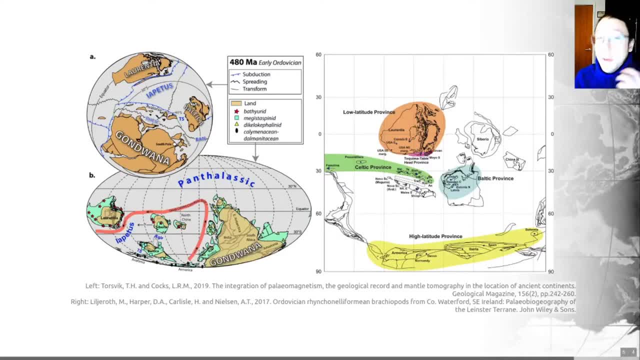 us to actually show in quite a bit more detail, beyond the mere existence of this ocean, what different continents were doing during different periods of geological history, And this is a story that's often told in terms of a three plate model. Within this model, we have oceans separating three continents, each of which is associated. 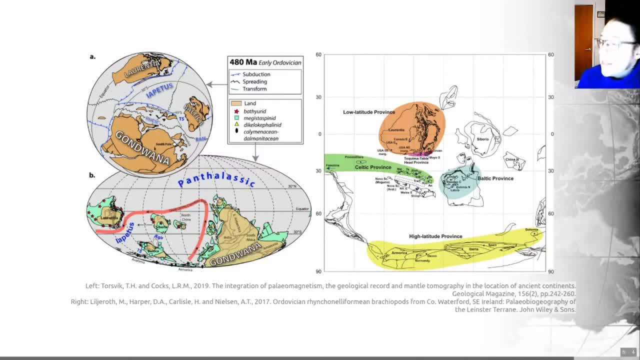 with a plate. These continents are called Gondwana- This is a continent that was just around and touching the South Pole at this time- And two northern continents called Baltica and Laurentia. So those are three of our plates that were around at this time and then there. 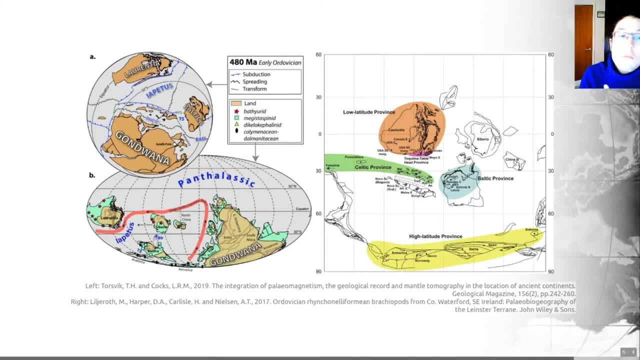 was another small bit of continental crust called Avalonia, And you can see which is labeled on this map here Now. this Avalonia broke away from Gondwana during the late Canvian to the earliest Ordovician period and, together with Baltica shown here, headed north to 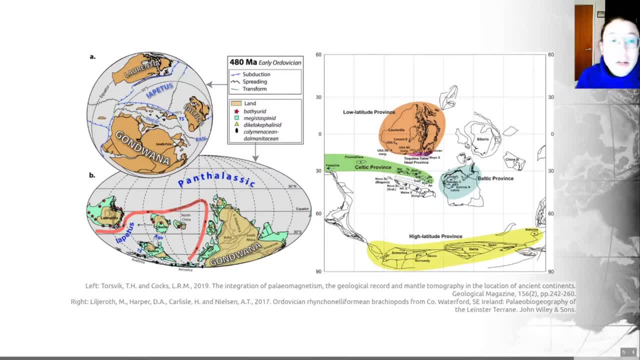 towards Laurentia. And we can tell that because it's a picture that's built up from faunal provinces. So on this image on the left-hand side here, you can see some examples of early Ordovician trilobite zones. So you can see there's a 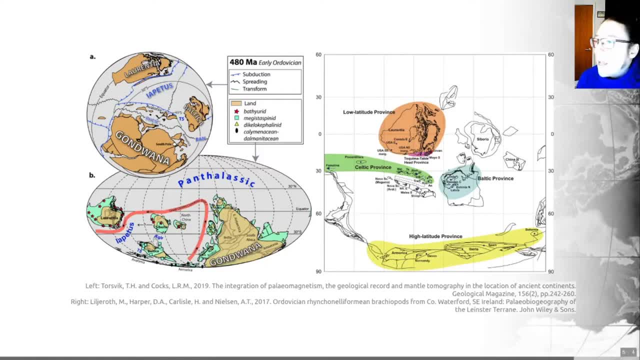 Mediterranean province called a Calaminacean or Delaminatician- Oh, there's a lot of long words in this one, I'm afraid Basically black circles shown here which occupied the continental shelves around the higher latitudes of the massive southern continent of Gondwana. We can also 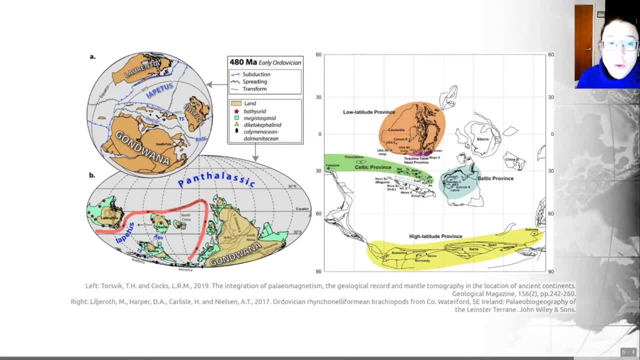 identify a Baltic province, otherwise known as the Megistanasped province. These are the light, blue or cyan squares here which are associated with Baltica and are nowadays found largely in northwestern Europe, And this was at temperate southerly latitudes. 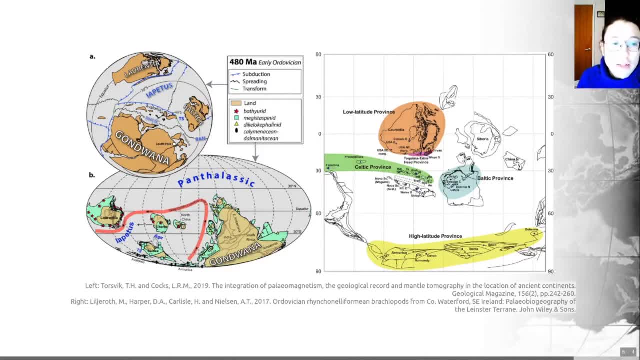 Oceans in the lowest equatorial latitudes hosted two distinct and separate faunal provinces. The first is the Bathyruid province- These are the red stars that are shown on this map here: Laurentia and Siberia and bits of China, And a separate Dichelokephalinid province- that one was difficult- which colonized the. 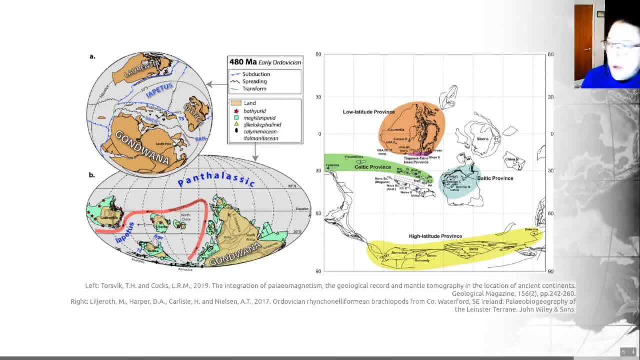 seas surrounding the margins of the lower latitude parts of Gondwana, So you can see those here. So this series of different associated species of trilobites kind of mark out provinces, each of which is associated with a different continent. during this, 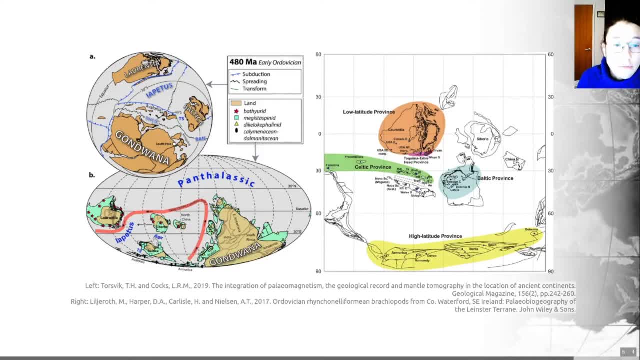 time period some 480 million years ago. The fact that we've got two different provinces at the same paleolatitude indicates that the ocean separating Laurentia, Siberia and North China, ie these red star continents and the large sector of Gondwana where we've got these yellow triangles, must have been large. 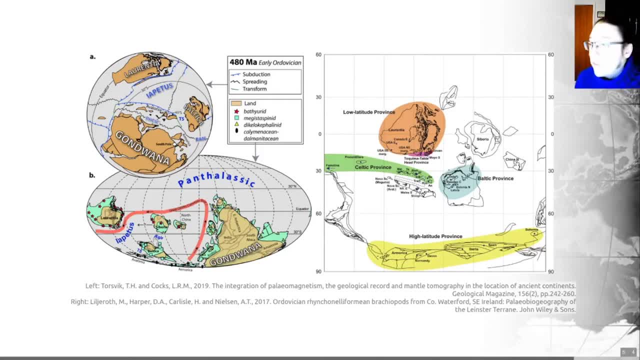 enough to have prevented the trilobite larvae from successfully crossing them. So these oceans here were probably smaller than this one. here is what we think. Provinces such as these are also reflected in the brachiopod fauna that we have from around. 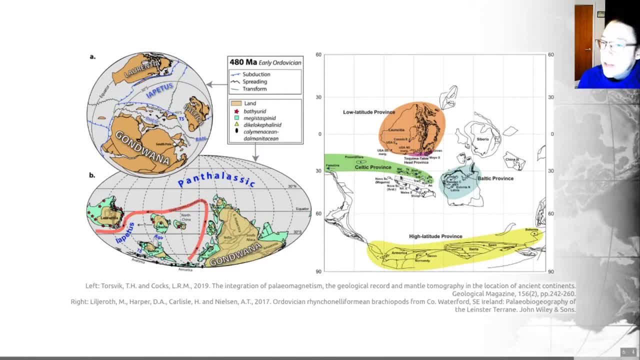 this time. So this is shown on the right hand side here and you can see that we've got four, five and indeed maybe even six different provinces in this time period. Those are probably the things that we need to study as we move forward. 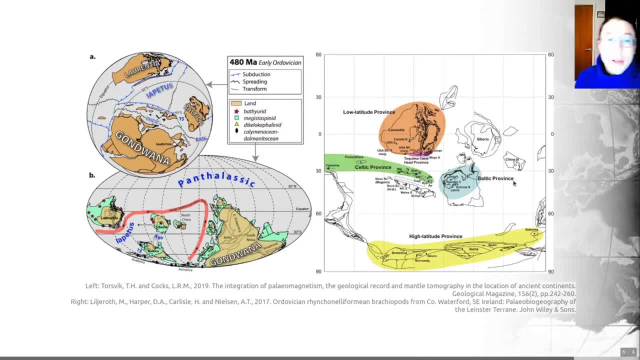 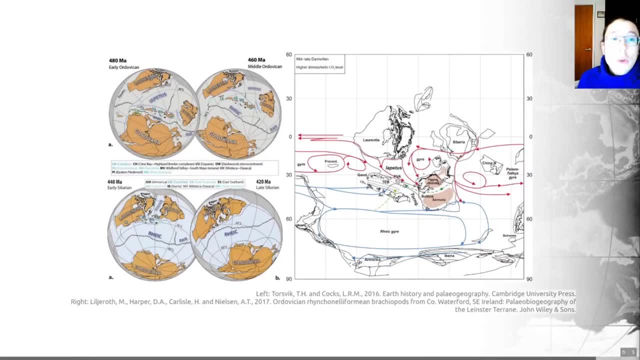 Uh, that's too much material. Let's go back, Let's look at the left over here and see if- and this time in our brachypod populations- so we can get really a good level of detail. We know. go further than that, though. we know there were also. 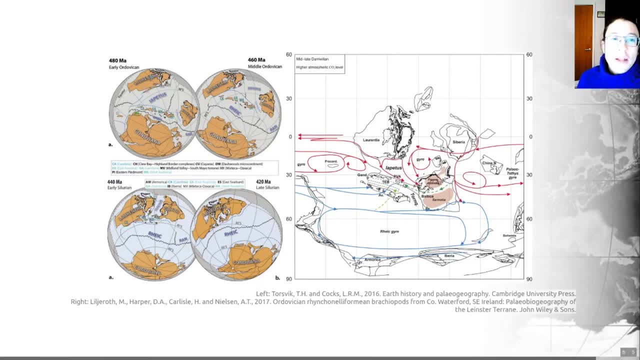 islands in the Arctic Ocean which were identified through peculiar faunas which we don't see elsewhere. So these are shown in the top left here, 480 million years ago. each one of these little islands shown moving northwards as time progresses is marked with its own little label. And so what we 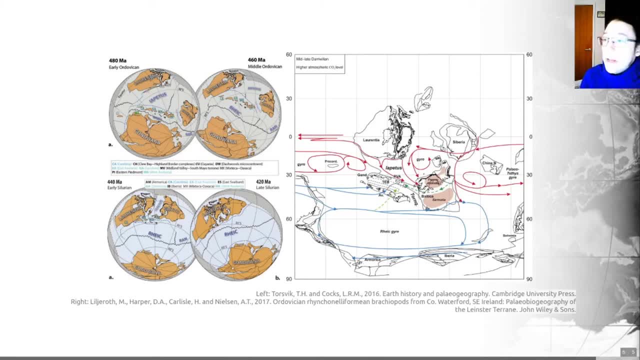 think happened, based on the fossils, is that Baltica moved northwards and as it did so it spun anti-clockwise, moving towards the equator and picking up these various terrains on the edge of its continent. So between 460 and 440 million years ago, all these little spits of land with their own fossils smashed. 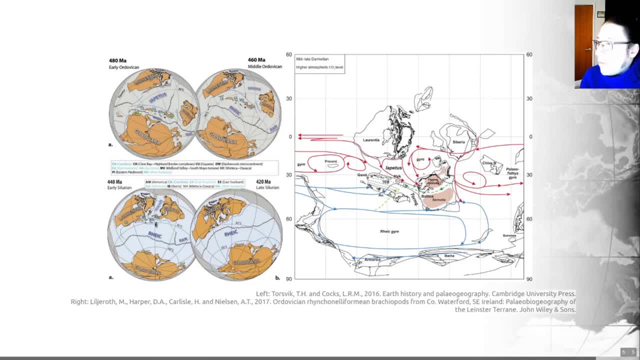 into Baltica, as you can see, a continent. So this is a very interesting example of what we can see in the Arctic Ocean. So we can see that this is the Arctic Ocean which we can see occurring by 440 million years ago, So by the late Silurian shown here. you can see that these continents had docked. 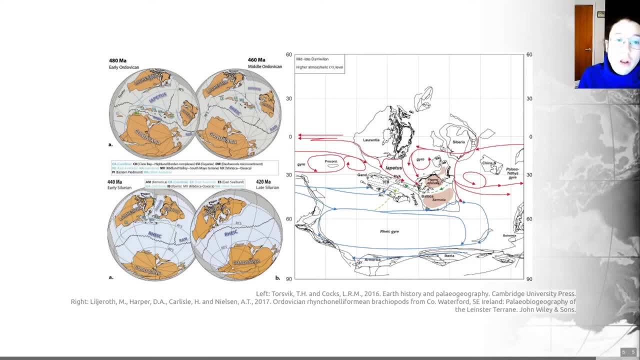 to formula Russia, this big northern continent. By the Devonian period, faunal provincialization had reduced in trilobites because this group was less diverse, but in contrast the brachypods had greatly developed, and the evolution of this ocean are largely based on the. 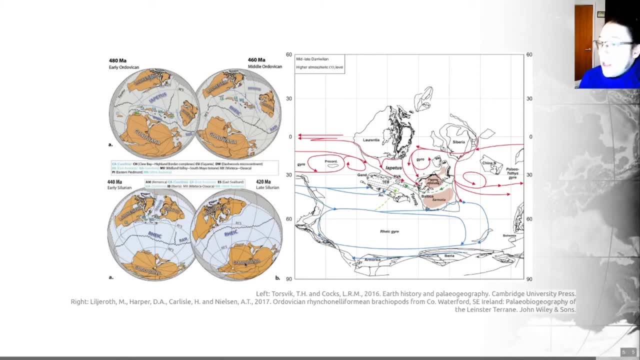 brachypods. After this point shown in the late Silurian, eventually Gondwana and La Russia collided to form Pangea, that supercontinent upon which the dinosaurs ultimately lived. And that's, that's a cool story, right, We can say a, really. 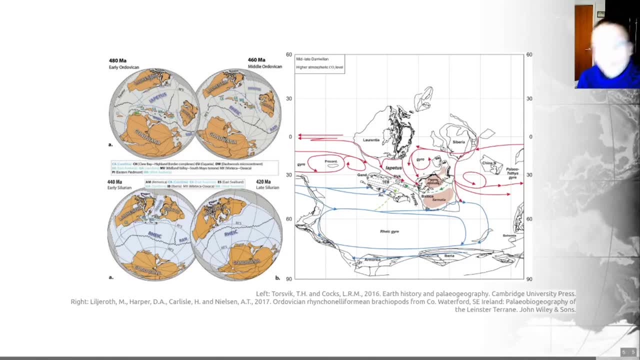 impressive amount of things from the fossil communities that we find associated with these ancient continents, But we can go into more detail into this in the next chapter. a step further, and reconstructions of the iapetus ocean system have all have even allowed us to. 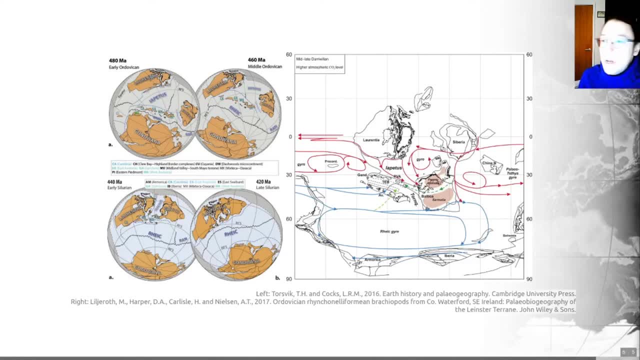 start mapping ocean currents and upwelling zones. so i've put an example of this on the right hand side here. that was created using a general circulation computer model based on paleo geographic maps. in this kind of this model of the ocean at this time, red and blue arrows represent 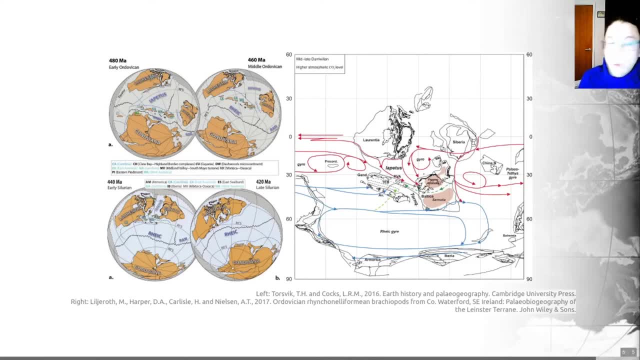 warm and cold currents respectively. all of this aids our understanding of possible migration routes of some key fossil groups during this time period, but those currents may, of course, impact on the distribution that we're seeing in the fossil record of these organisms. for example, the distribution of low latitude and warm fauna may have been influenced by strong and persistent 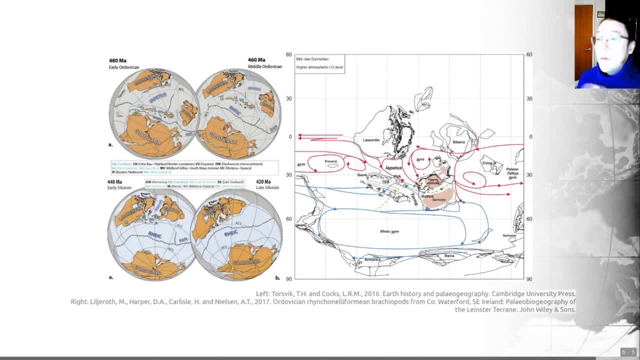 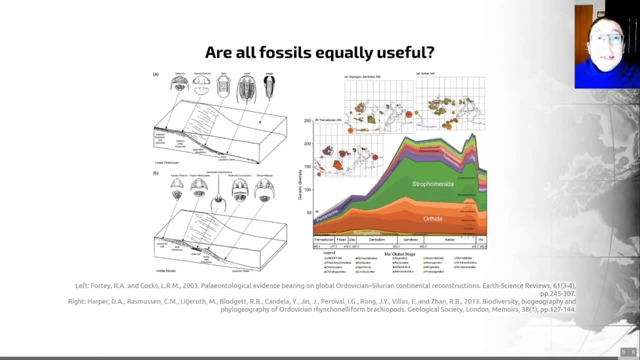 warm ocean currents. so that's another thing we have to bear in mind when we're trying to better understand what was going on in deep time. so, in summary, to reiterate, the early paleozoic biogeography that i've just shown you builds on an analysis of trilobite and sessile brachiopod. 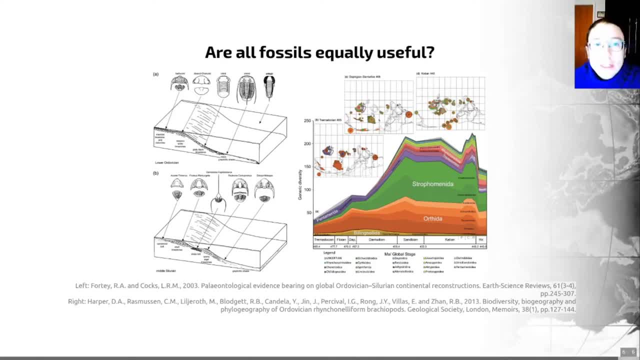 distributions, sessile means attached to the sea floor. these are an example of our success and as these diagrams show. so, for example, this is lower ordovician to middle silurian in terms of the changes in um in trilobite communities, and on the right hand side we can see a series of ordovician um changes. 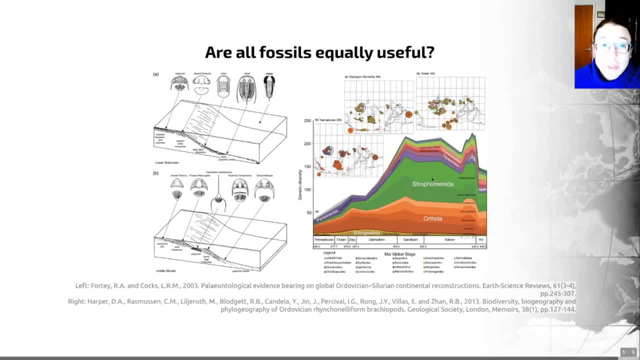 in terms of the diversity of different brachiopod groups. as you can see from those um, communities change in time as well as space and, as you can imagine, with this kind of dynamic it gets very complicated very quickly. there are lots of different factors we have to consider, including 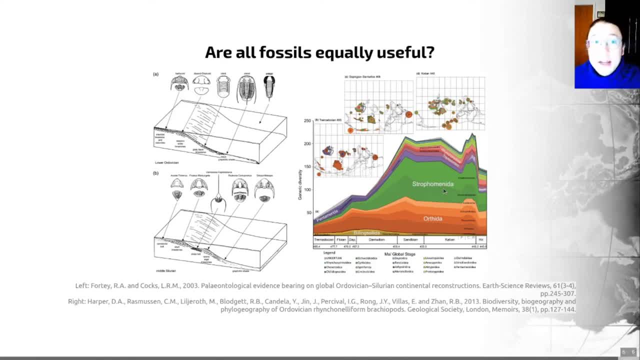 climatic changes, as well as the space, as we're looking at the future of the ocean, and the future of the ocean as we're looking at paleo biogeography, and a key question then is if we're using these fossils as a tool to understand biogeography in the past. are all fossils as good? 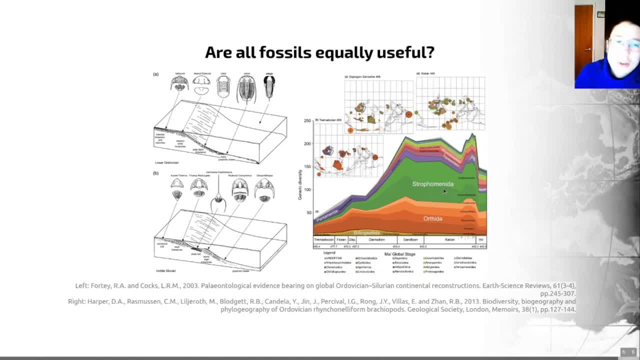 as each other for biogeographic analysis, or do we have bad and good fossils when it comes to biogeography? as a living example of a good um organism for biogeographic analysis, the polar bear would be a very good example, because it has an obvious and well-defined biogeographic range. 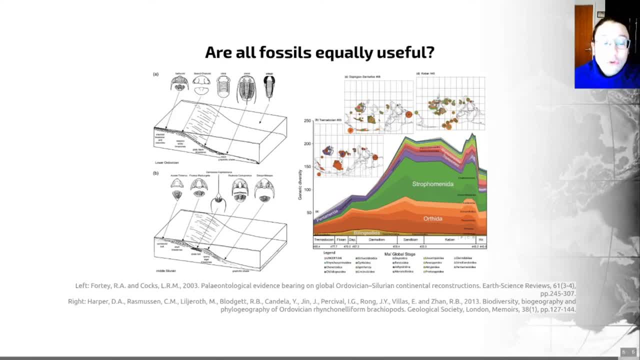 that's not true of all organisms today, and it's certainly not true of all organisms today, and it's certainly not true of all organisms today and it's certainly not true of all fossil organisms- and a number of key conditions must be satisfied if fossil data are to be effective when describing past um geographies, for example. 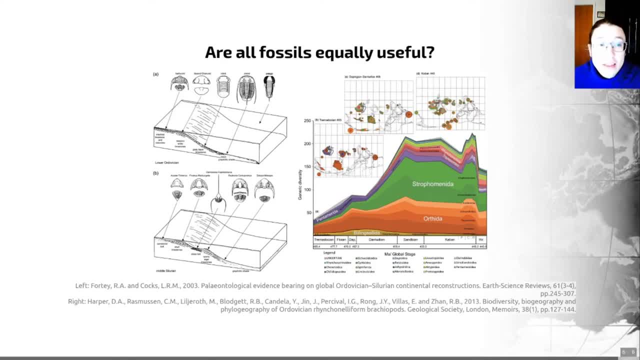 we almost always need to know the precise age and, ideally, the lifestyle of organisms in order to help us use them as tools for building a biogeography. in terms of organisms that are planktonic, pelagic or nektonic, ie those that float or swim, those will have a distribution. 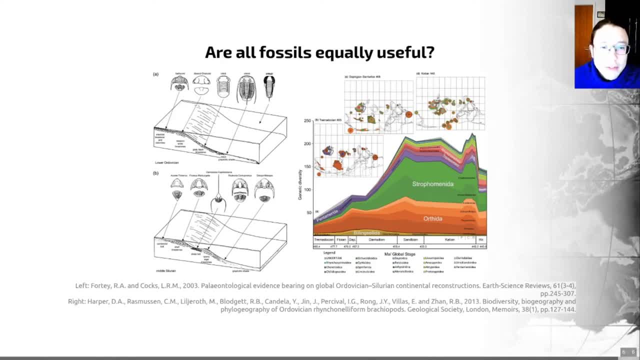 that's controlled by the movement and the temperature of water masses. as such, they may be of latitudinal significance, ie we find them in belts, but they will usually not be related to particular terrains, so a terrain being a fragment or block of continental crust with its own. 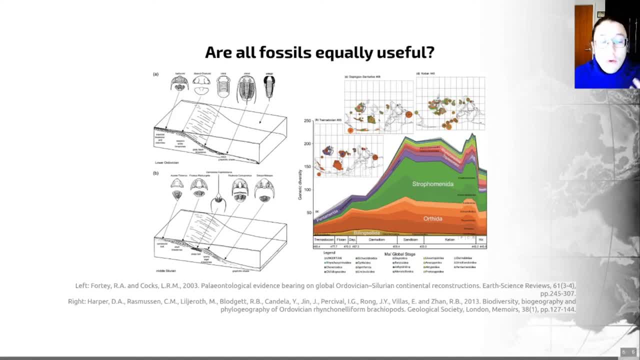 individual geological history. rather, we see those terrains within benthic organisms or those that swim near the bottom, so these are organisms that are living on the sea floor or just above it. we see, indeed, within these communities, provinces associated with domains at shallow depths, but with increasing depth, these generally become, these organisms become more cosmopolitan. 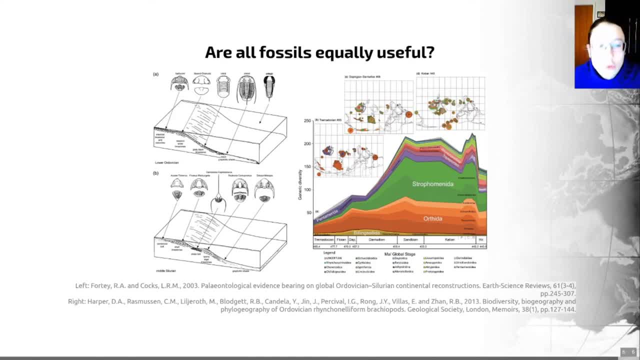 so that's because conditions at depth are generally more uniform, with regards to temperature and substrate, than in shallow water, so there's less provincialism as a result. exceptions do exist, especially within deeper ocean regions, but these organisms are generally more cosmopolitan, and so these are all considerations we have to factor in to paleobiogeographic continental reconstructions. 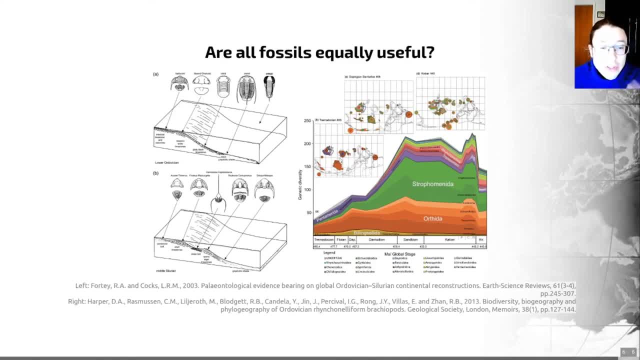 and when we're building these reconstructions, these analyses, we need to be aware of the ecology of the organisms that we're looking at and we need to compare fossils with similar lifestyles and from similar facies- so i'm found- of similar kinds of rock- to try and exclude ecological and environmental effects as we're considering our 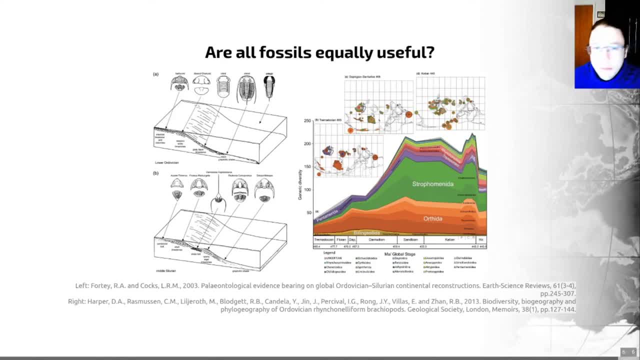 paleobiography. and that brings me to the end of my example that's based on the iapetus ocean. i will be featuring a few more slides as part of our zoom session, looking at patterns of biodiversity and taking those into deep time. so that's another element of paleobiography, but until then, i hope.